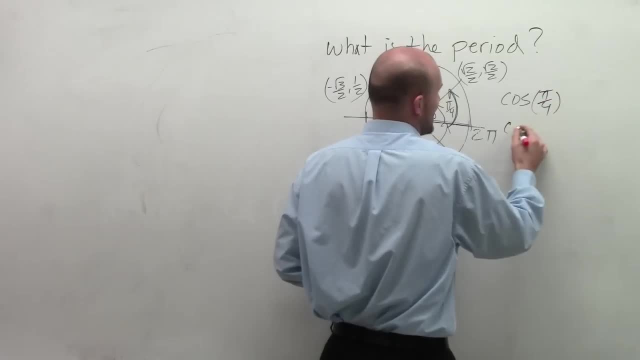 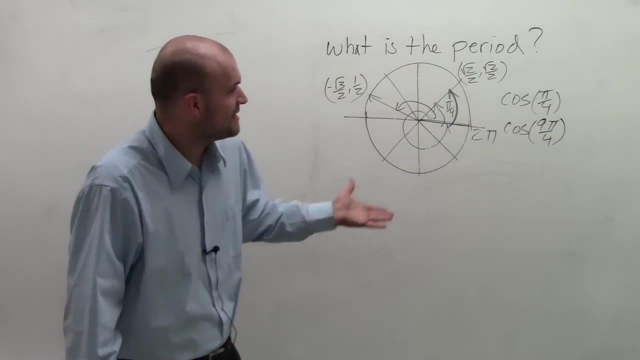 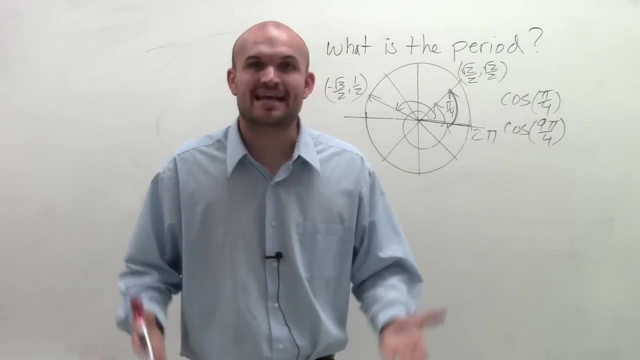 the cosine of pi over 4 is exactly the same as the cosine of 9 pi over 4.. And the same thing. even if I went around again, if I kept on adding 2 pi, we're still going to get the exact same values. It's just going to. all we need to do is just add again. 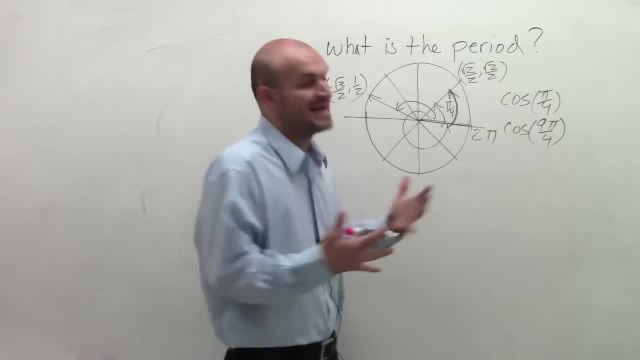 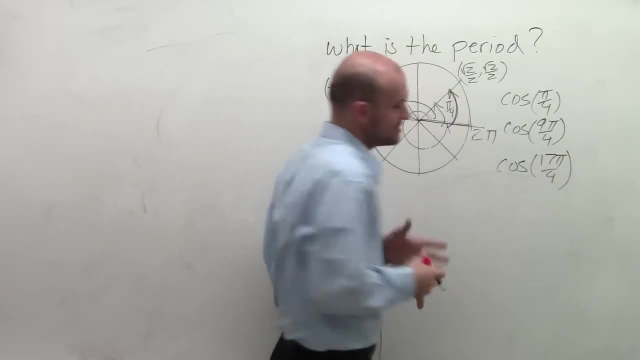 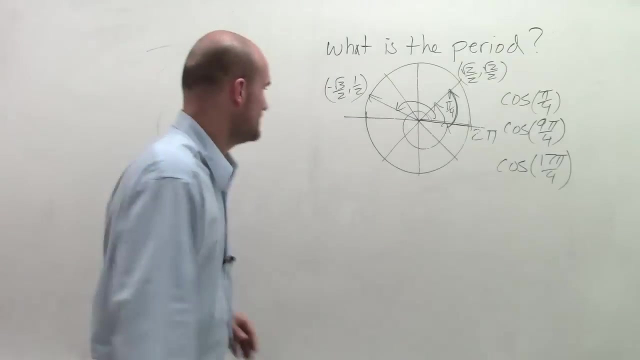 another 2 pi and we're going to get back to our exact same point again. So if I say the cosine of 17 pi over 4.. And so what happens is our graph repeats itself. Even though we have different output values, we're getting the exact same output values. 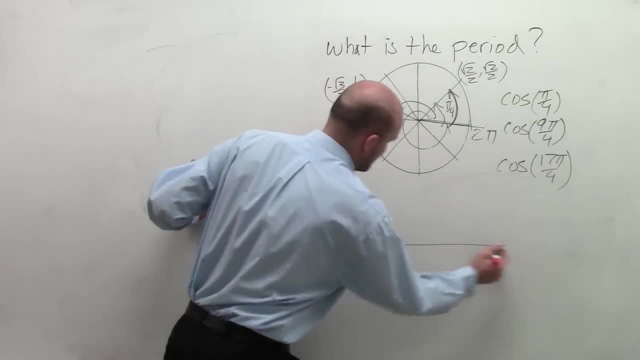 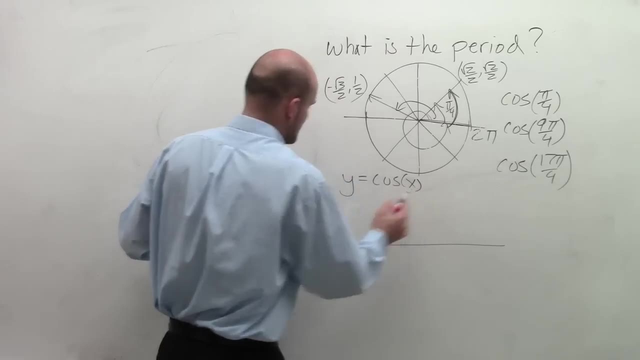 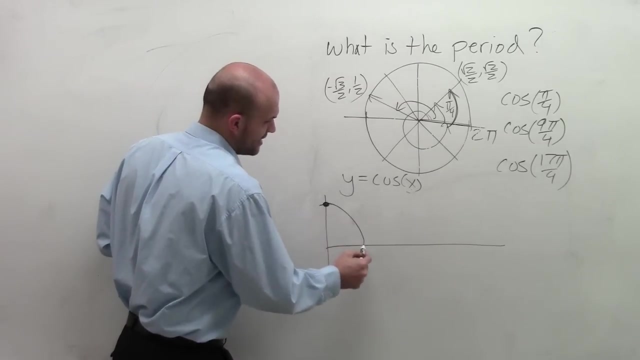 So when we're graphing- and I'm just going to utilize the cosine function here- So y equals cosine of x, All right. So when looking at the cosine graph- and we can do this- the same thing for the y, But when we look at a point, we start at 0.. And then our next. 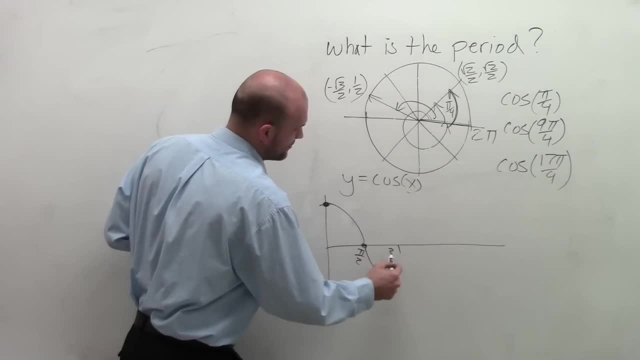 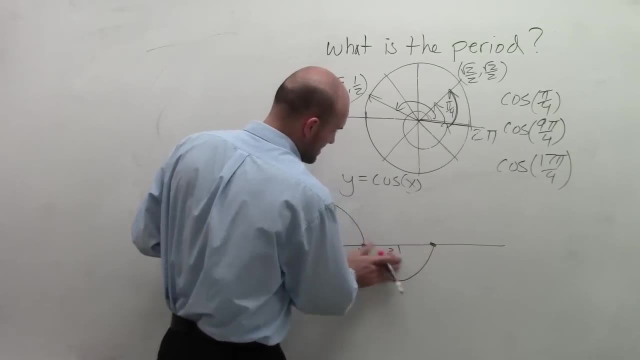 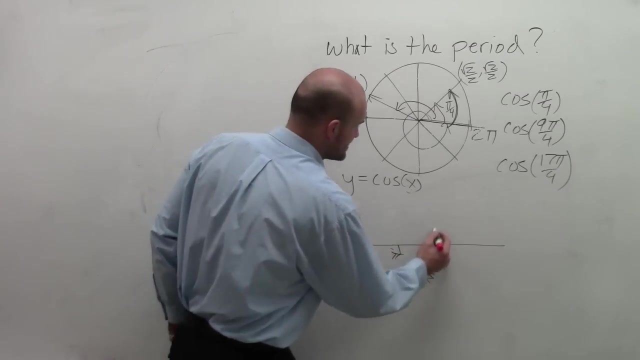 point is: pi half, We have 0. Then we go down at 3 pi halves. We're down at negative 1. And then we come back up to 0 at- I'm sorry that's- at pi, And then at 3 pi halves. what we do is we come back up to 0. And then at 2 pi we're. 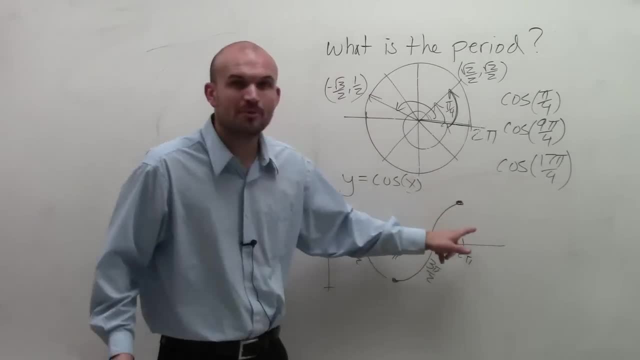 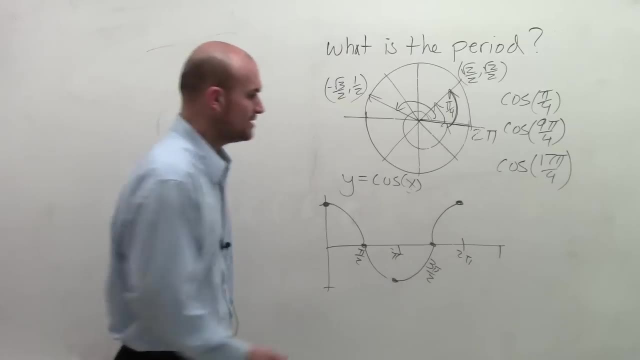 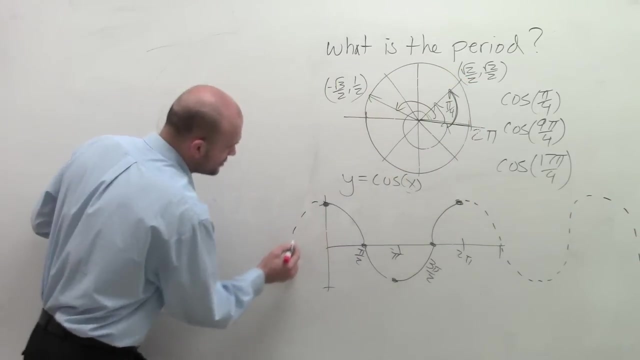 back up to 1 again And what you notice is from 0 to 2 pi. I'm at the exact same point where I started, And if I was to continue this for more and more points, what you'll notice is the graph continues to do the exact same pattern. So what asking is: what is the? 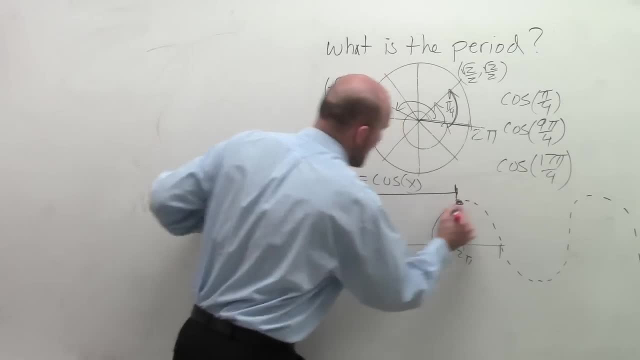 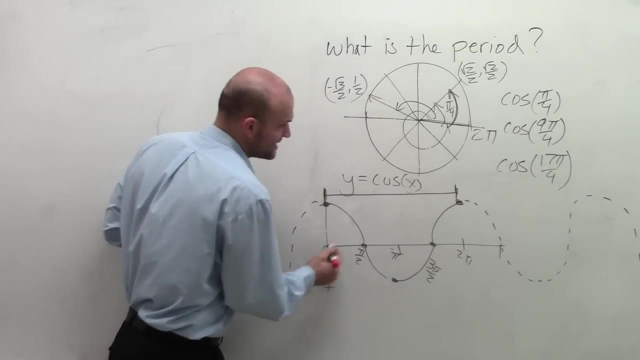 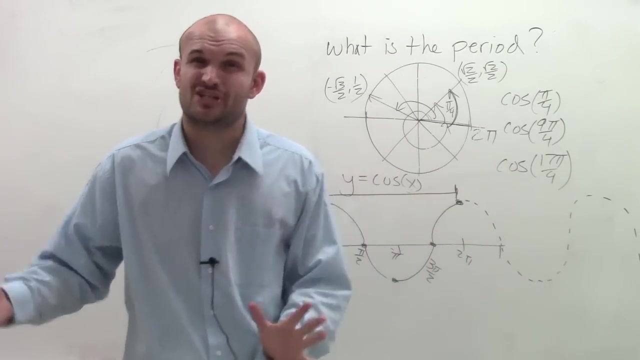 period. What is the distance? The distance that a graph takes before it starts repeating itself. So for sine and cosine, that distance is 2 pi. Now, how do we figure that out? How do we always know? Is it always going to have the same period? Is it going to change? How do we know exactly what it's? 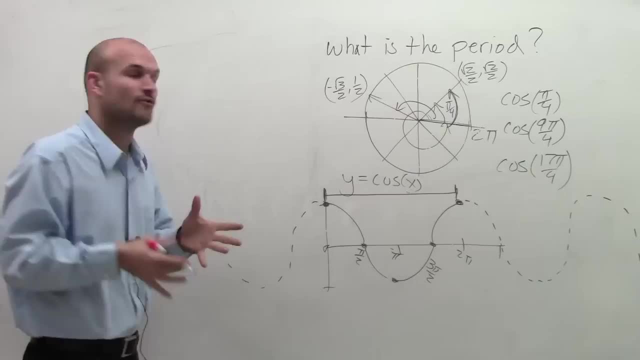 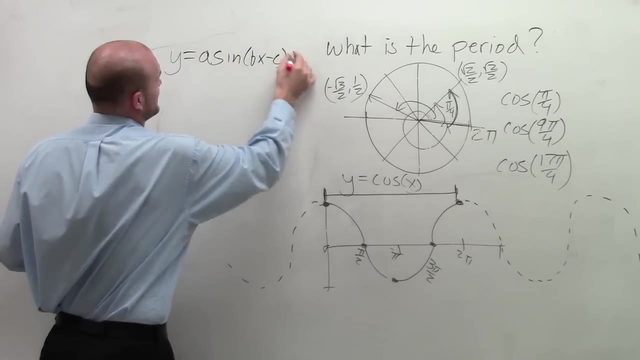 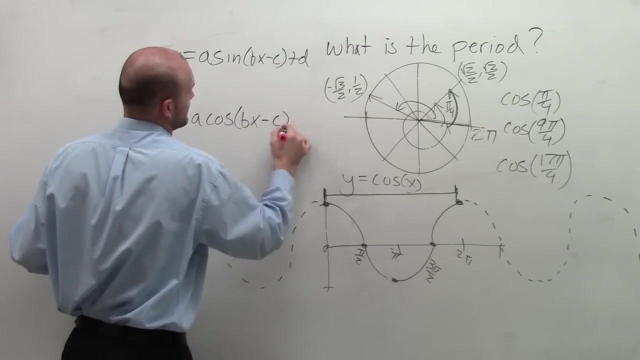 going to be or what it's going to be Well, to do that, we need to look at our standard form for each function. So we have y equals a times sine of bx minus c plus d, And we know that we have y equals a cosine of bx minus c plus d. And what we notice is when 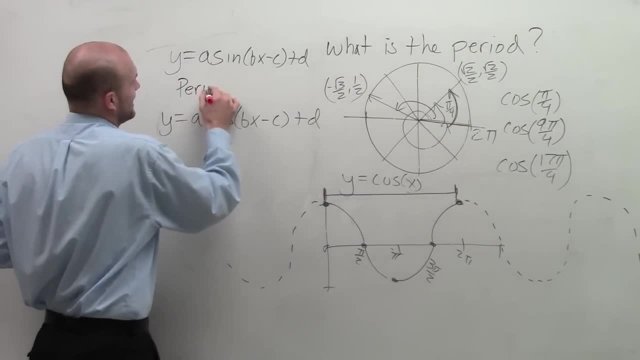 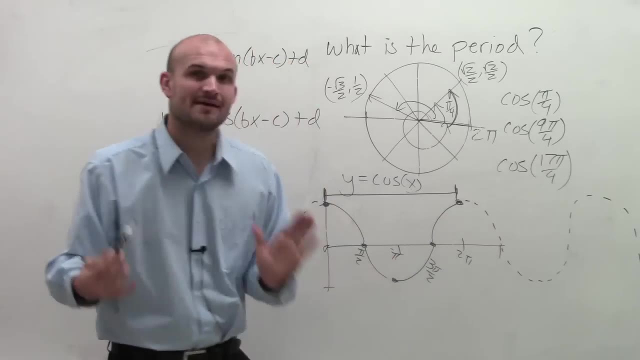 trying to determine the period. what we're going to do is the period is going to be affected. So we know that for cosine and for sine, this distance where it takes the graph to repeat itself- even though I only have the sine graph pictured- it's the same, exact same thing for 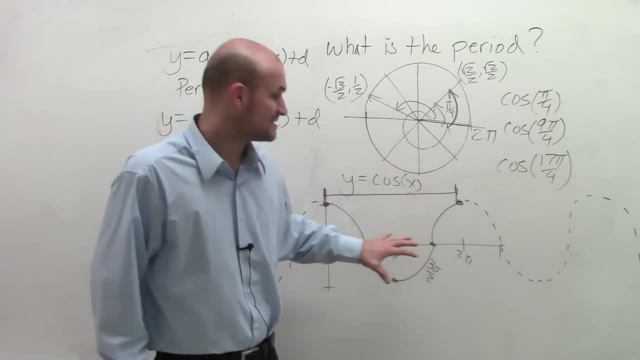 the sine, or I only have the cosine graph pictured. It's the exact same thing for the sine graph, But this distance is 2 pi. So what we're going to do is we're going to practice the cosine graph, And what we're going to do is we're going to practice the sine graph And we're going to. 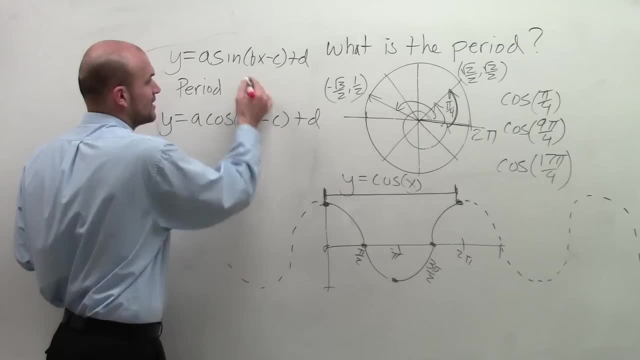 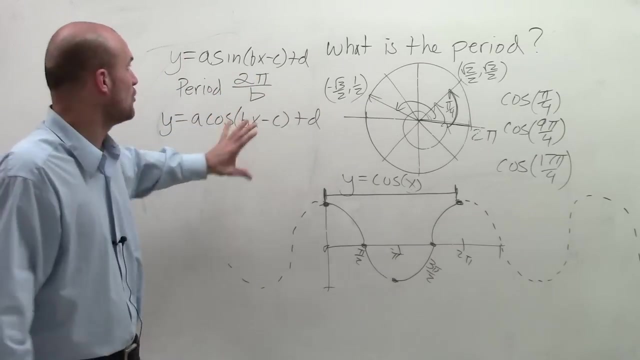 So you can say: the period of all sine and cosine graphs is going to be 2 pi, unless you have a alteration or a transformation of b. So if you have a number that's going to be in there for b, you're going to take 2 pi and divide it by b And that works for both sine and cosine graphs. 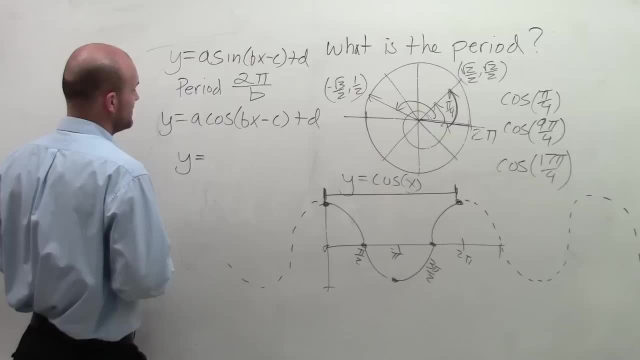 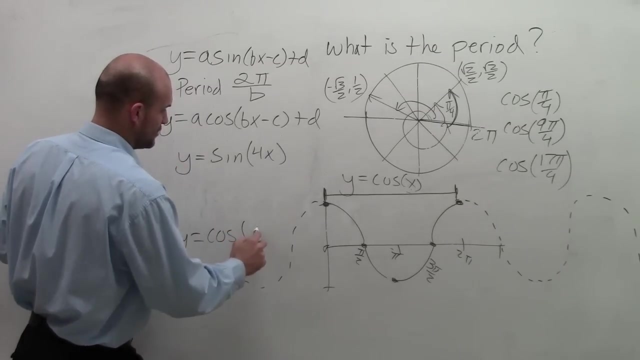 So let's just take a look at you know kind of two functions here. Let's say I have y equals the sine of 4x And then let's do y equals the cosine of, let's do the cosine of pi divided by. 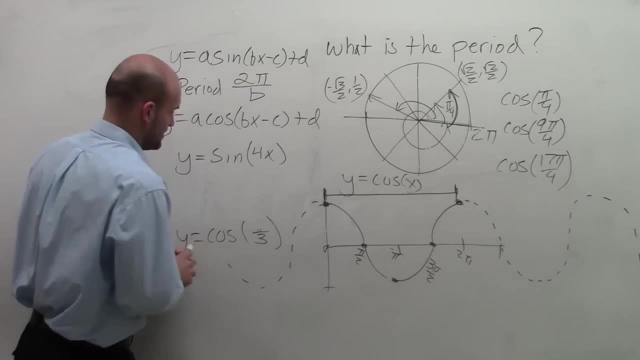 3, all right of x divided by 3.. Okay, So in this case, what we need to do is we need to determine what b is in each instance. So in this case, we have a value of b which equals 4.. So, therefore, 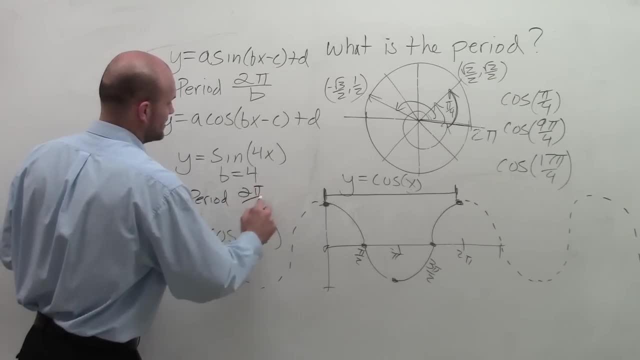 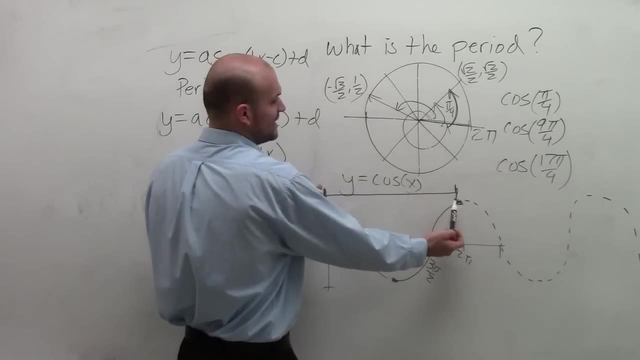 my period is going to be 2 pi. 2 pi divided by 4, which equals pi halves. So that means, rather than the distance of my graph competing a cycle at 2 pi. now my graph is going to complete a cycle in the distance of pi. So you: 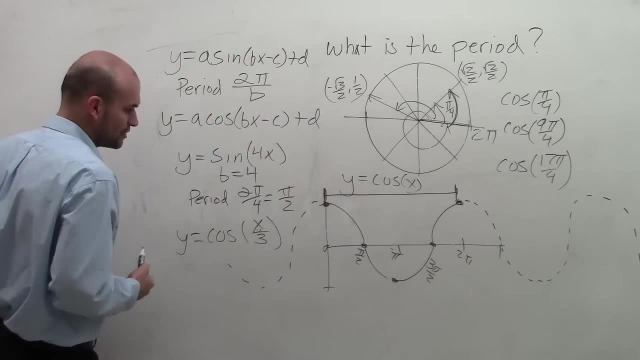 can see it's been shrunk. Now, when I look at cosine of x over 3, I can determine that b is equal to the value in front of. x is 1, 1 being divided by 3.. So therefore it's equal to 1 third. 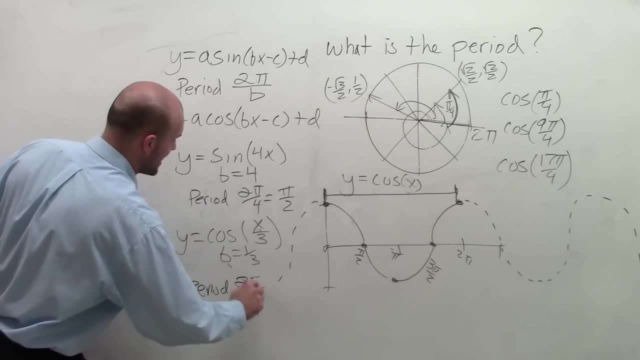 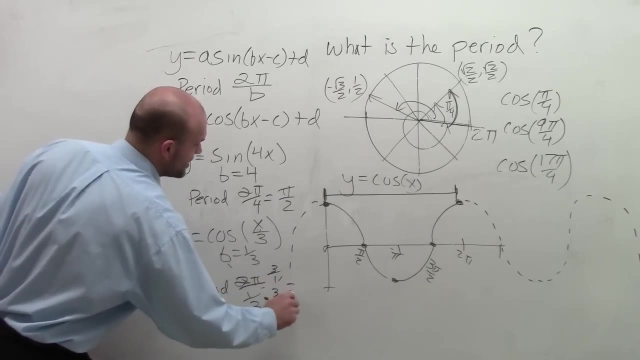 So my period is going to be 2 pi divided by 1 third, And to divide by a fraction, we multiply by the reciprocal And therefore I get a period of 6 pi. So therefore, if I was going to graph this, 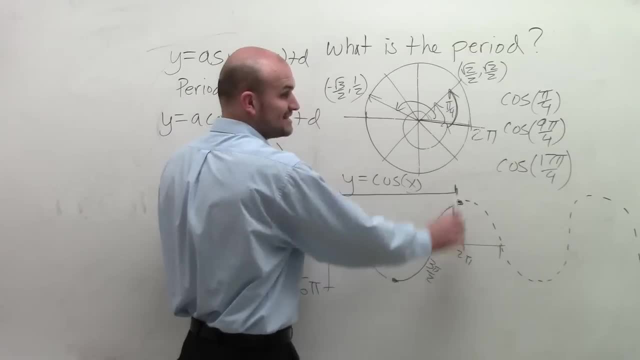 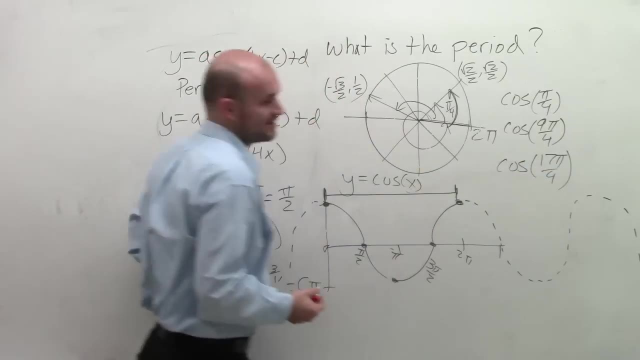 function with a period of 6 pi, rather than it taking a distance of 2 pi for the graph to repeat itself. it's now going to take a distance of three times what I'm showing you for the graph to complete itself. So it's being stretched horizontally. So there you go, ladies and gentlemen. That is.